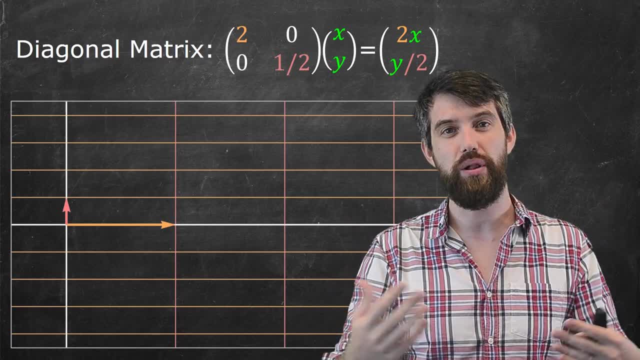 stretching of 2 in the horizontal and stretching by a half in the vertical, and then diagonal matrices are also nice because they're really easy to visualize. So I'm going to take this diagonal matrix and I'm going to subtract the two parts and I'll give it aした five, so that 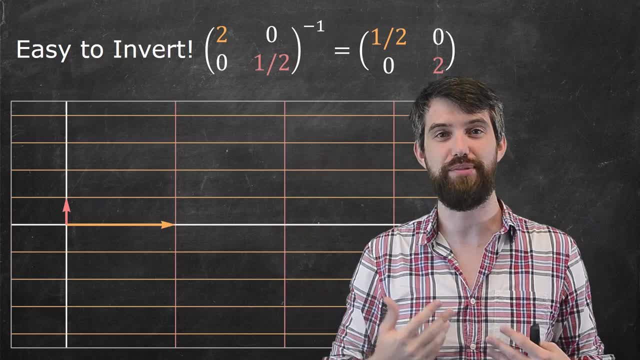 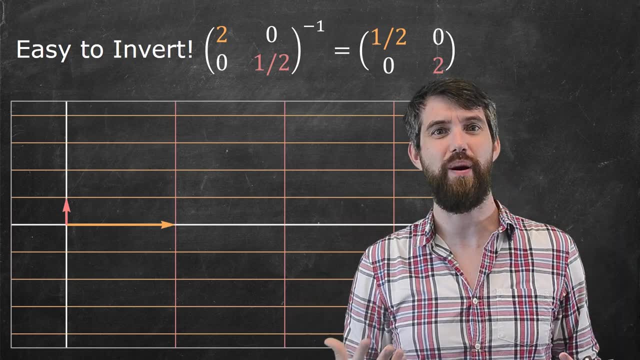 I can also take the 3 and subtract the 2, and subtract the half, and subtract the half over them. so this is the matrix 1, half, 0, 0, 2. and then, if I think about what that diagonal matrix does, well, it takes the horizontal parts and it squishes it by this factor of half and it stretches by a. 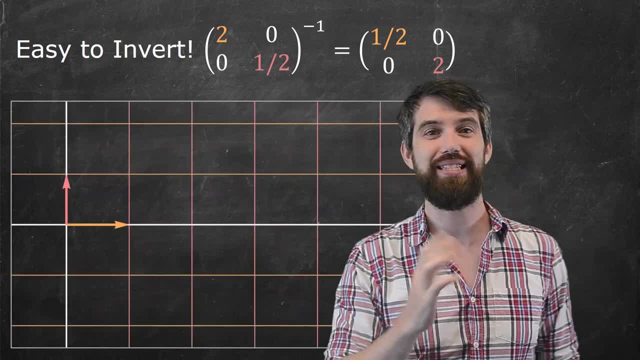 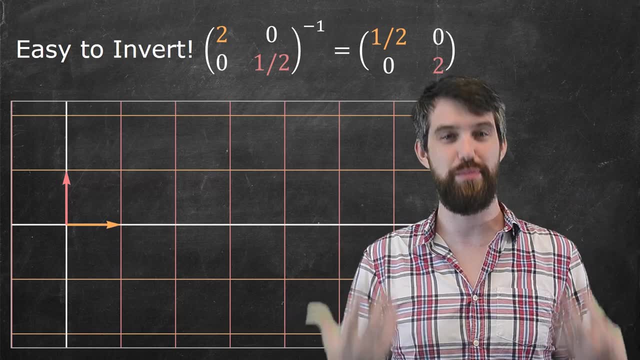 factor of 2 the vertical parts, and we get something like this, taking it back exactly where we began. Alright, so that's pretty nice. and, in fact, diagonal matrices. you could think of them in very large numbers of dimensions and you could kind of visualize them to. 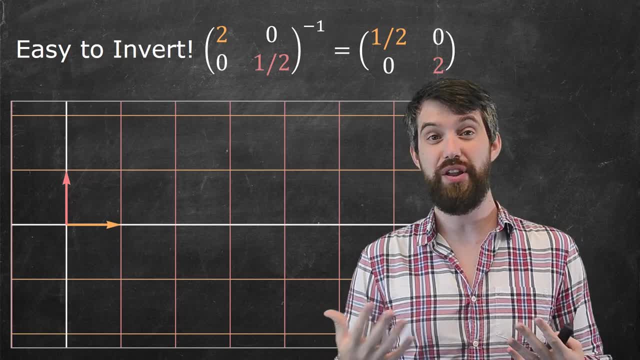 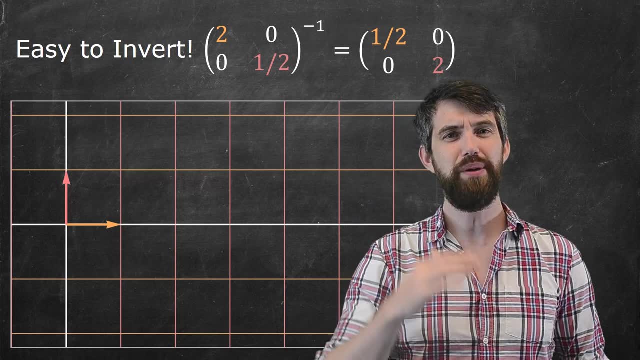 something like this: So now you've got a square matrix with a diagonal-like matrix and you get a extent by saying whatever axis you happen to be on, then you're going to stretch along that particular axis by whatever the scaling factor is of that component along the diagonal. But what? 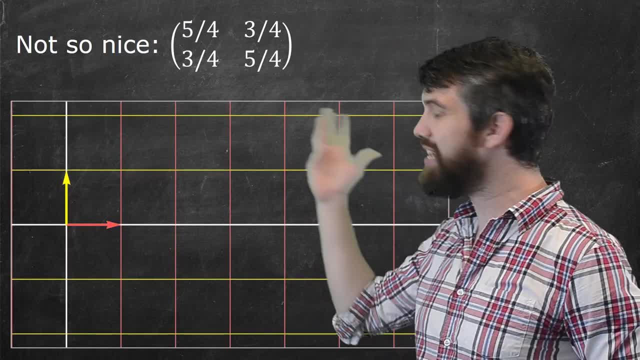 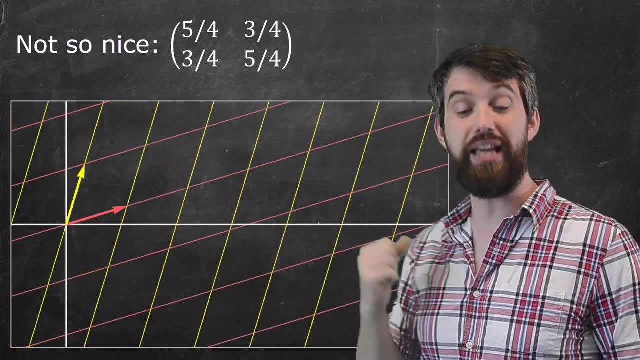 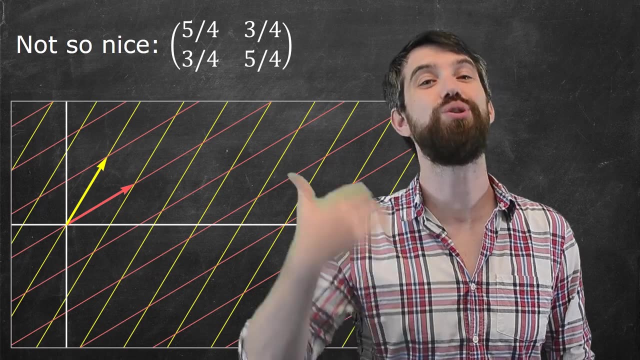 about a matrix that's not quite as nice. How about this one here? Now, it's not that I can't visualize this. Indeed, I can visualize this particular matrix. It's going to look a little bit like this: That is the 1,- 0, the first basis vector went to 5 quarters, 3 quarters and 0, 1, the second basis. 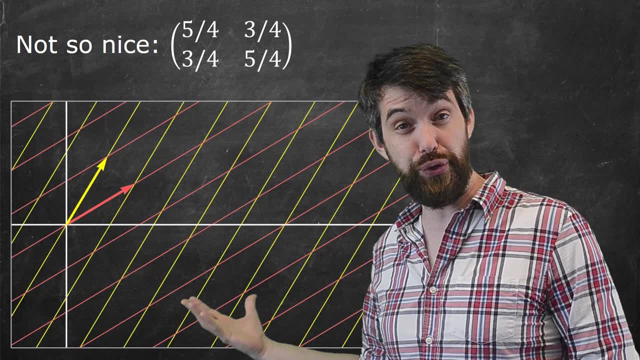 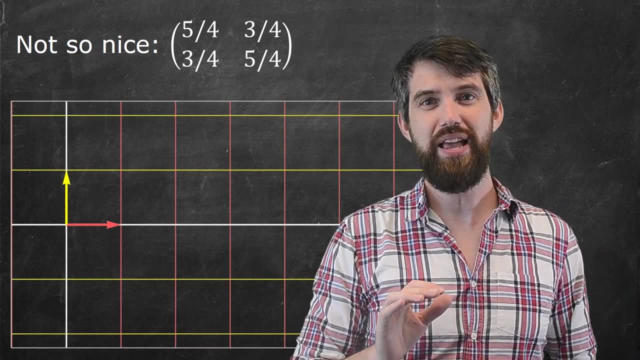 vector went to 3 quarters, 5 quarters, So I can indeed visualize it, but I think it's just a little bit, messier. Let's watch it one more time. I start in this sort of nice standard basis and then all of my grid lines. they both get closer together and they're going to move around, They're going. 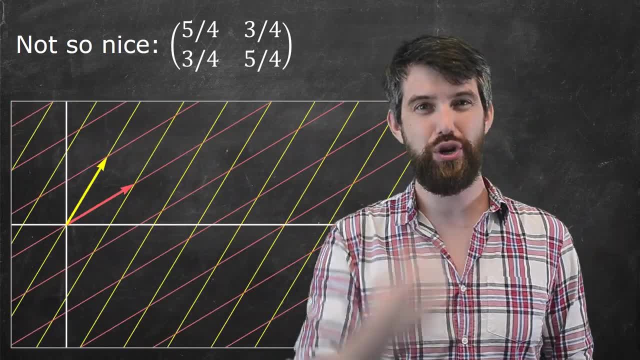 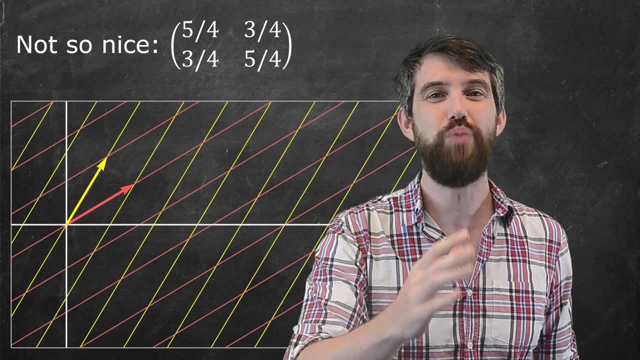 to transform. So I can do this in two dimensions and visualize it quite well. but if it was a large number of dimensions and all sorts of things were happening at the same time, it would be kind of hard to keep track of it, and that's why we want to deal with eigenvalues, eigenvectors, diagonalization. 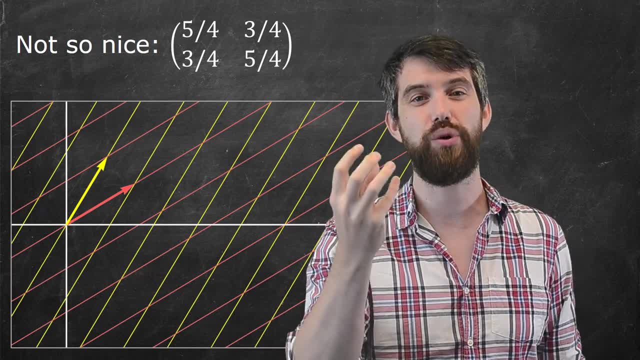 with the second basis vector. So that's why we want to deal with eigenvalues, eigenvectors, diagonalization with the third basis vector, want to think of complicated transformations in an easier way, So let's go and look at the eigenvalues. 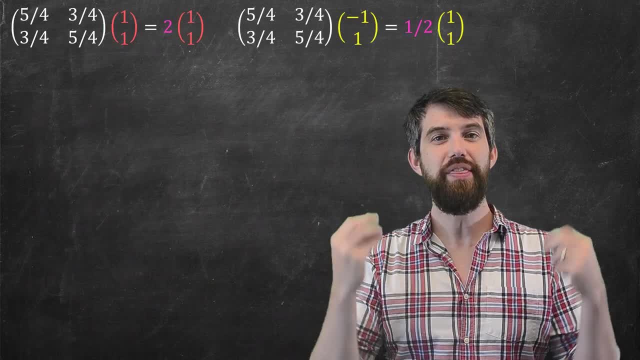 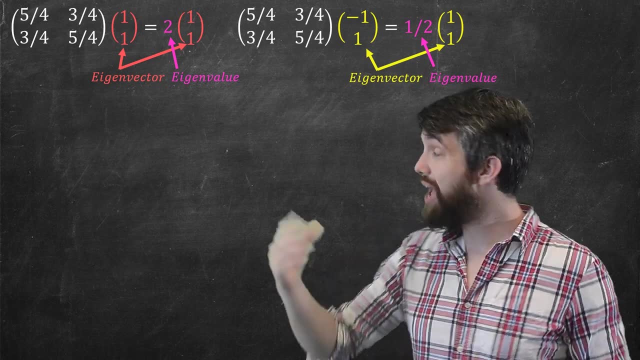 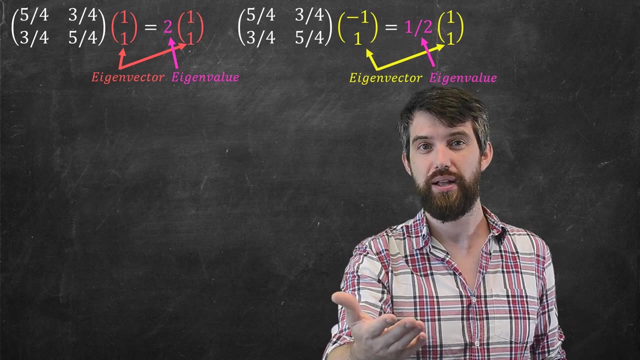 and eigenvectors for this particular matrix. Here they are here and these give me these eigenvalue eigenvector pairs. So, for instance, corresponding to the eigenvalue 2, I have an eigenvector 1, 1 and what that does is, when the matrix applies to 1, 1, it just multiplies that vector by 2.. 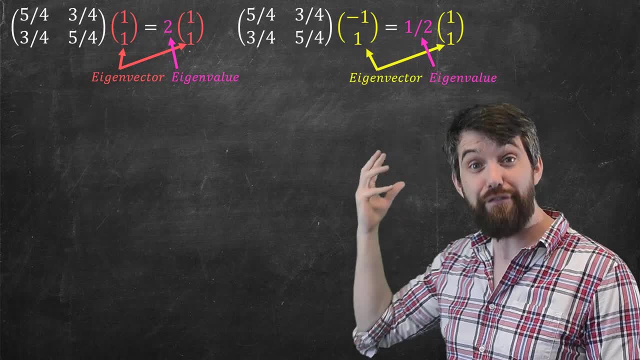 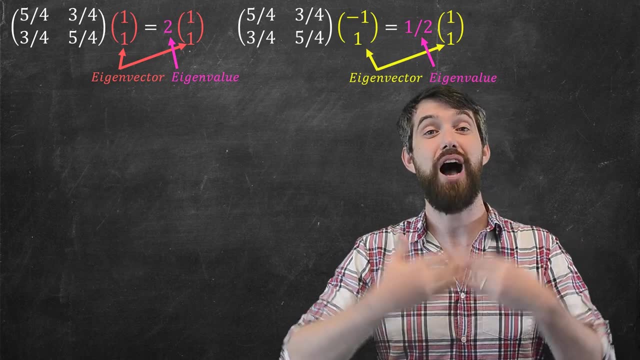 And likewise I've got this eigenvalue, the one half, and if I have the corresponding eigenvector minus 1, 1, when I multiply the matrix to it, it just stretches it by a factor of a half. There's this compression. Now I'm not going to show you how to come up with the eigenvalues and the eigenvectors. 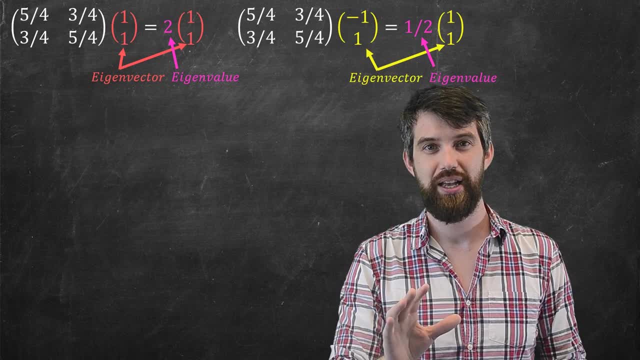 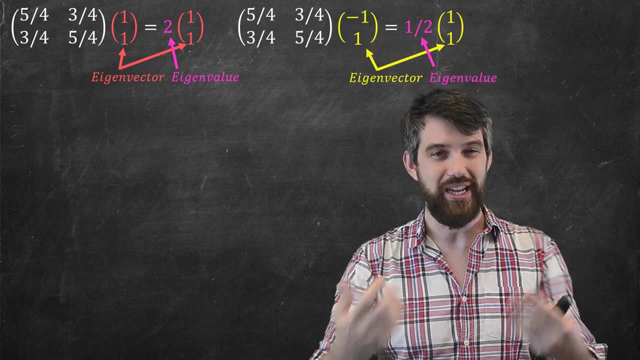 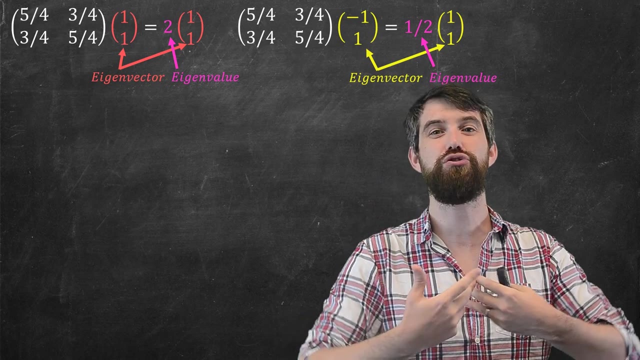 Algebraically. I've got a previous video for that. but the key point is this: When I look at an eigenvector, this is a direction where the matrix applies in a very simple way. It's just a stretching factor, kind of like we had with diagonal matrices. For diagonal matrices it was very simple with just stretching. 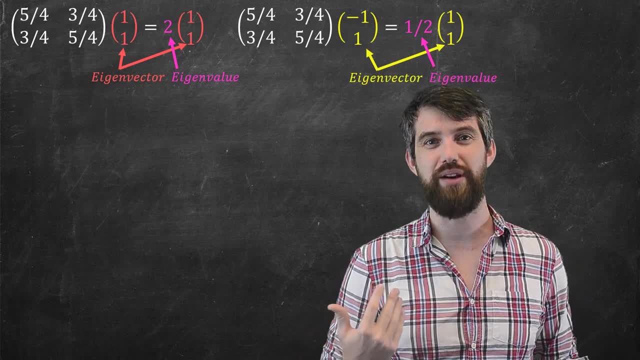 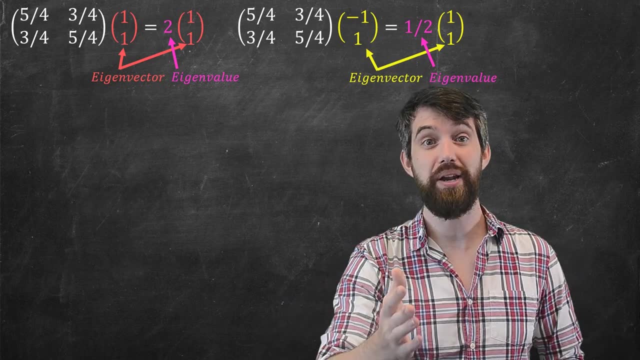 the standard basis vectors For eigenvector, eigenvalue pairs in those specific directions. the matrix just works by stretching as well. All right, so now let me draw the plane. but now I'm going to draw the plane where the grid lines, the coordinate system is going to come from these. 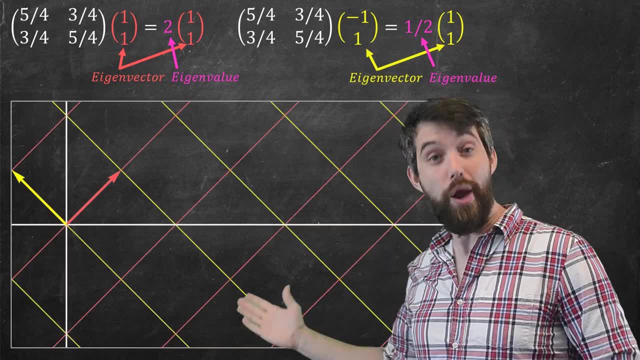 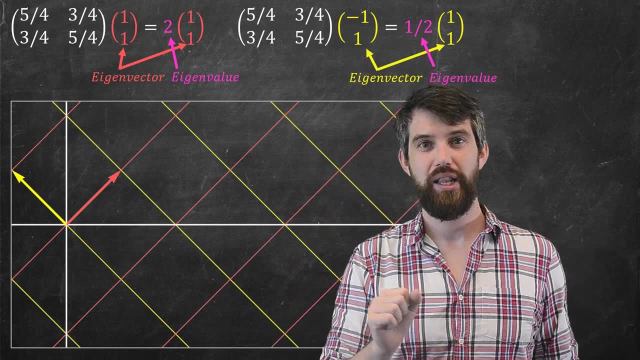 eigenvectors. So here it is, As in: I put in the 1, 1, the first eigenvector, I put in the minus 1, 1, the second eigenvector, and I've drawn a grid system that corresponds to it. Now I haven't. 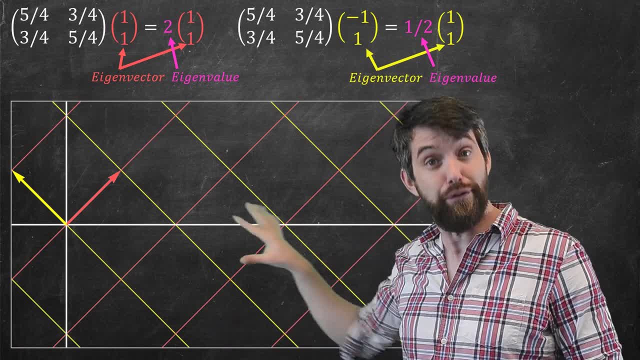 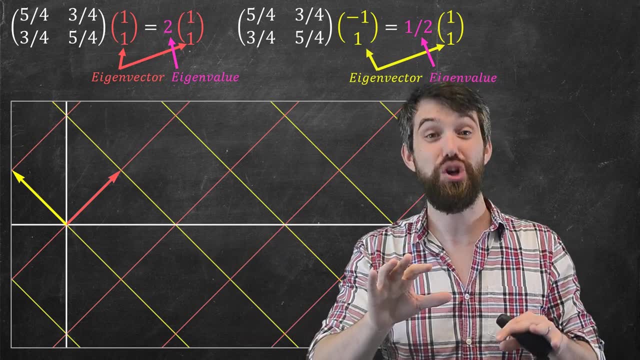 applied my transformation. yet Indeed, I've just taken a different choice of the lines that I want to draw on the screen. I could have drawn the standard basis lines, but I've chosen to draw these ones. All right, I'm going to show now how this particular 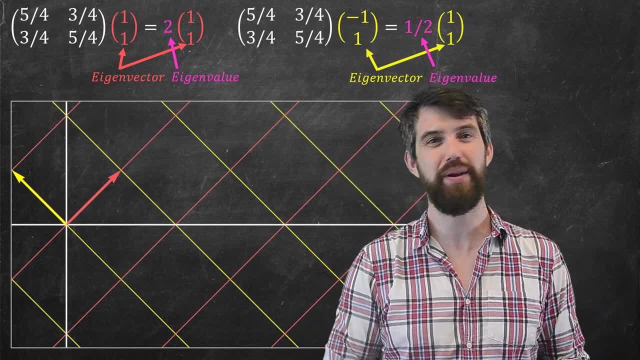 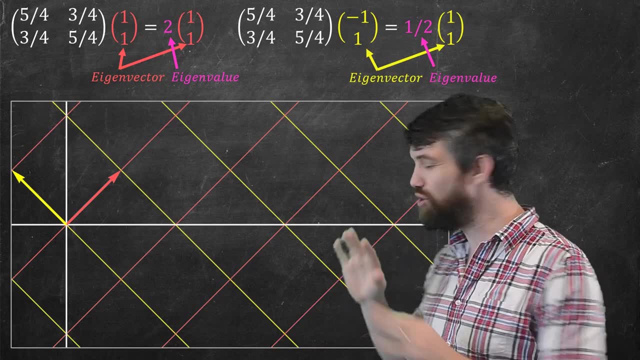 grid system transforms under the application of this matrix. but I want you to pause the video first and just think about it yourselves, That's all right, I'll just wait over here. You just pause, You think about how this is going to transform, All right. so here's the answer. It looks like this: 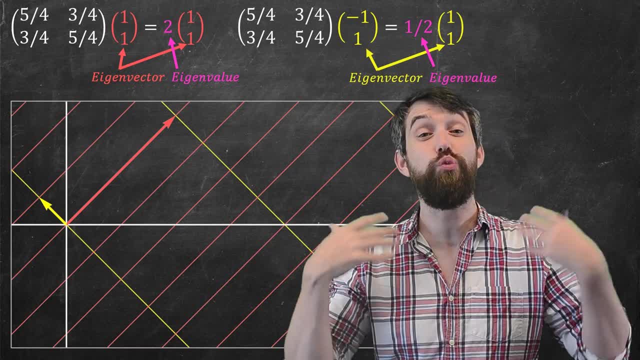 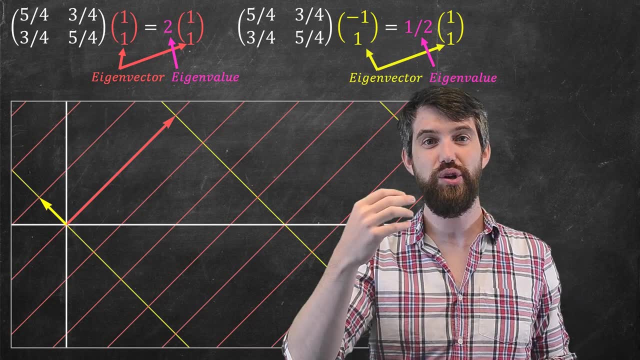 So what happened is that, if I looked at the yellow grid lines, which are originally began, separated by one copy of the 1, 1 basis vector. So what happened is that when I took the 1, 1 vector and it got multiplied by 2, the separation between the yellow grid lines. 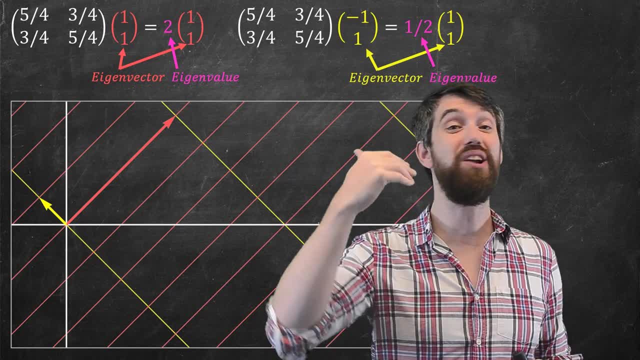 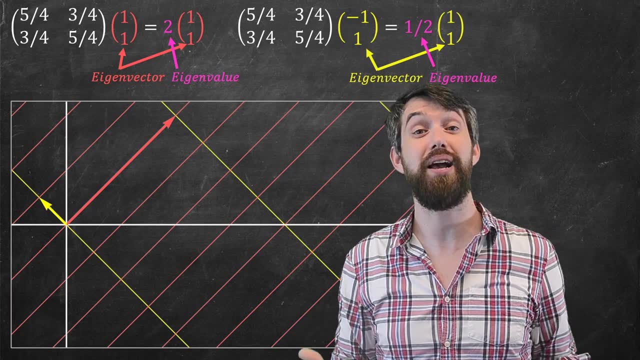 also got multiplied by a factor of 2.. All right, so what we've seen is that if I can go to eigenvalues and eigenvectors and I can write a grid system based on those, that sometimes my matrices can look a little bit nicer. But I want to go even further. Let's go and try to diagonalize a matrix. Now the 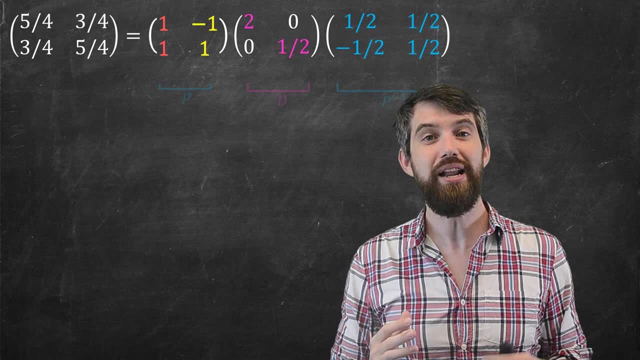 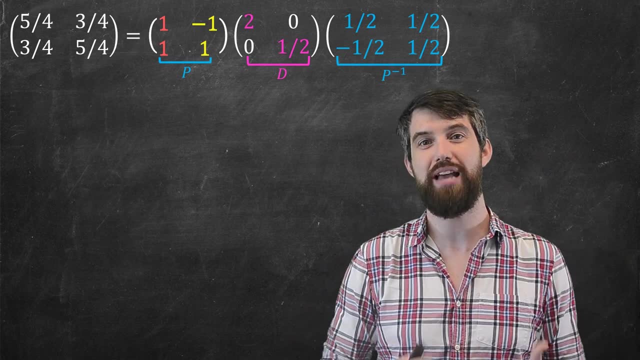 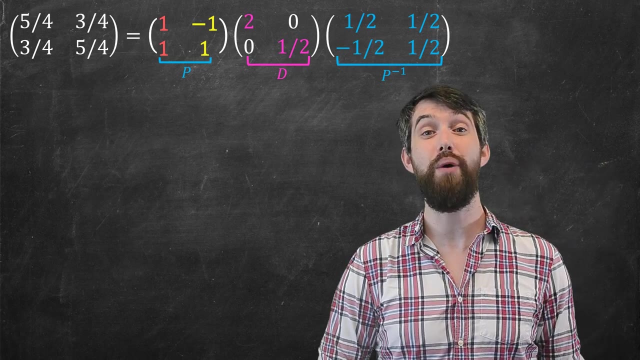 process is going to be this. So I've got a matrix and I've written it as a pdp inverse and I've got previous videos for that if you want to look into how I came up with that particular product and how to algebraically execute the computation to fill it in. But the key thing is this: We're just going to go and have for 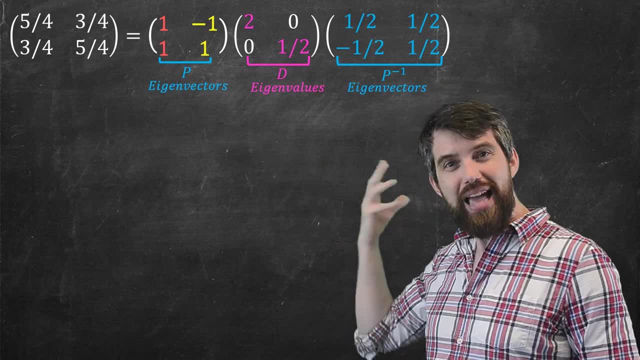 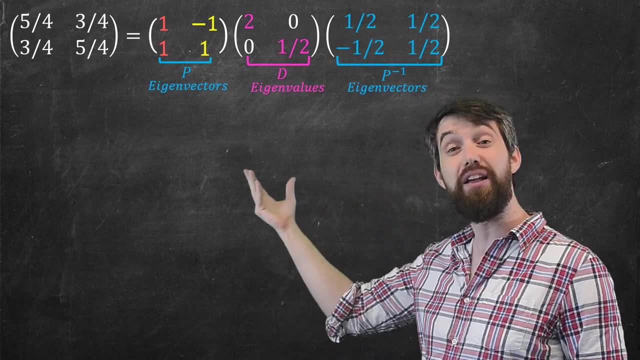 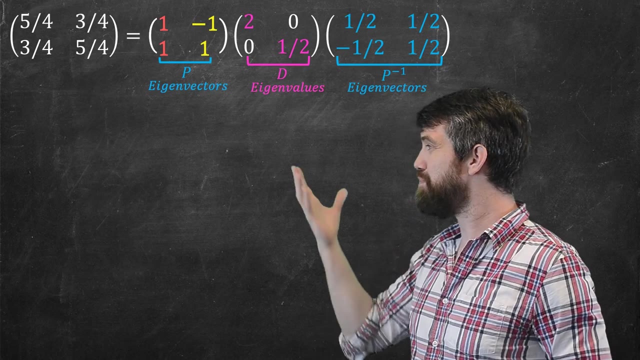 the p matrix, it's just going to be the eigenvectors. and then for the diagonal matrix, along that main diagonal, are just the corresponding eigenvalues, in the same order in which the eigenvectors appear in p, The inverse of that particular matrix. So what we have here is a product of three matrices, of which 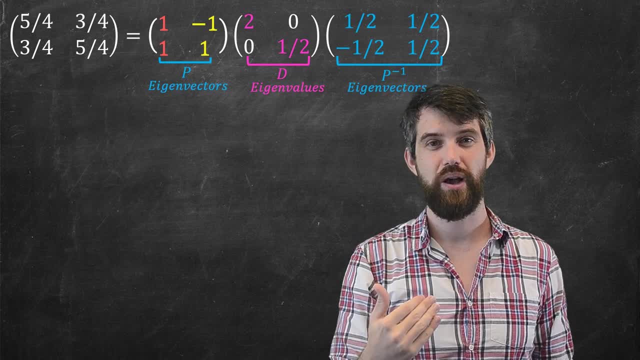 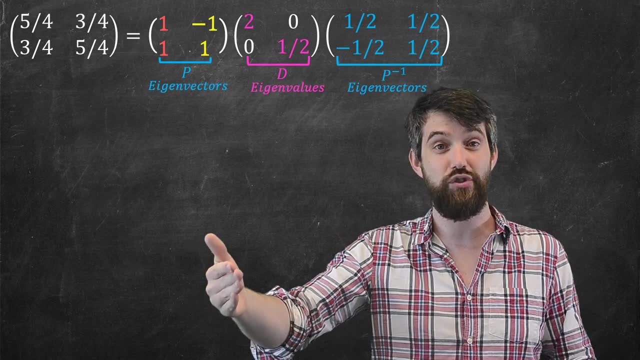 this middle one is a diagonal matrix. Okay, so our goal here is to try to understand this as some statement about transformations, A composition of three transformations that's geometrically going to go through stuff. We want to be able to trace that. Now I want to analyze this a little bit. 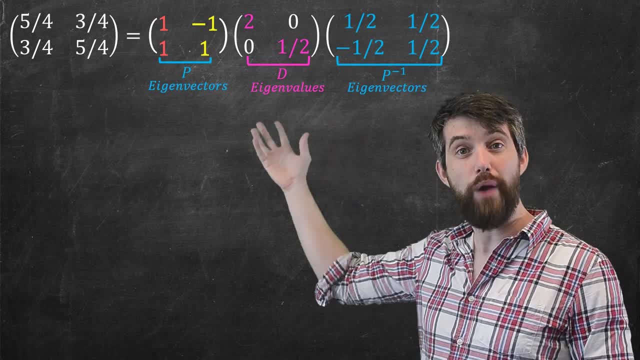 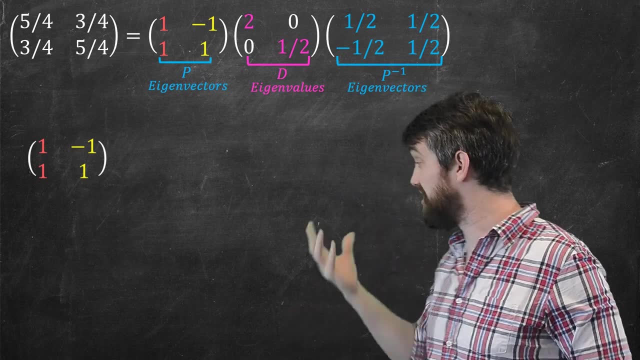 further. So the first point is: let me come up here and look at this 1, 1 minus 1 matrix. Now, if I take this matrix and apply it to any particular vector, like say c1, c2, what it does by the definition of 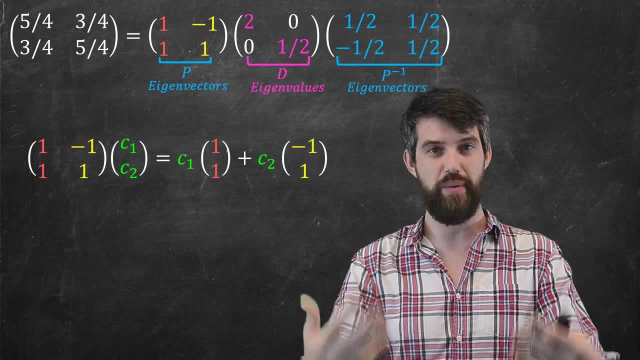 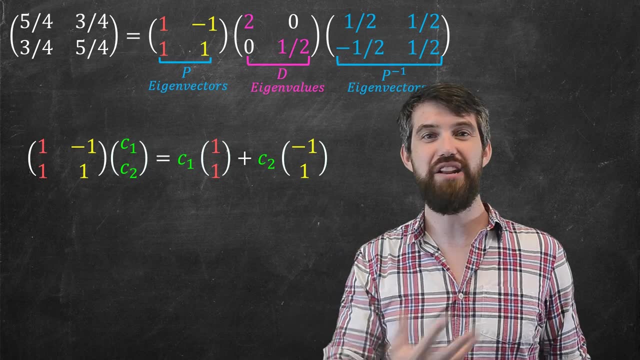 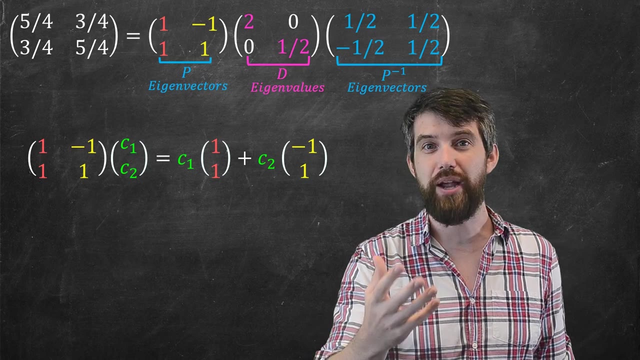 what multiplication by matrix is. it is taking a linear combination of the columns of this matrix, A linear combination, in this case, of the eigenvectors. So this is the kind of matrix we've seen as a transformation of basis. But what it does when we multiply by this particular p matrix? 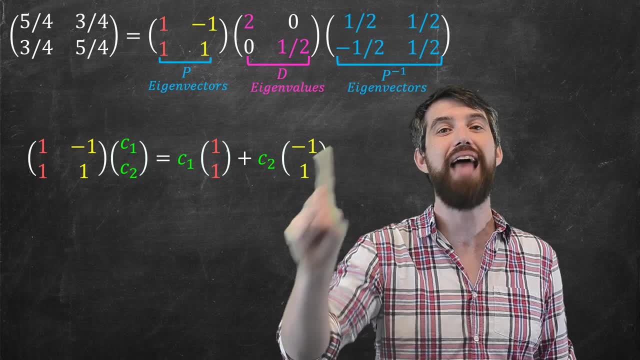 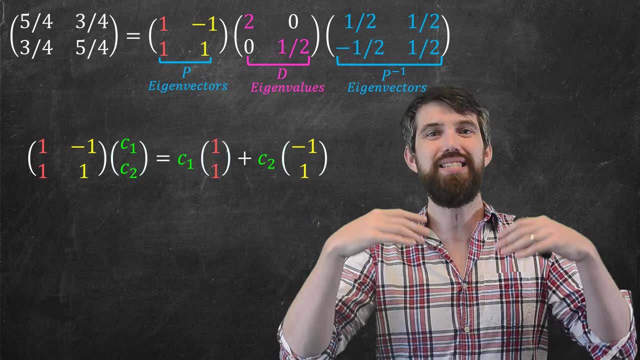 is it? it takes a vector- c1, c2- that is written in that so-called eigen basis- a negative basis of i vectors, and it converts it to the standard basis, That is, this is a change of basis matrix that takes vectors that are written in the eigen basis and writes them into the standard basis. 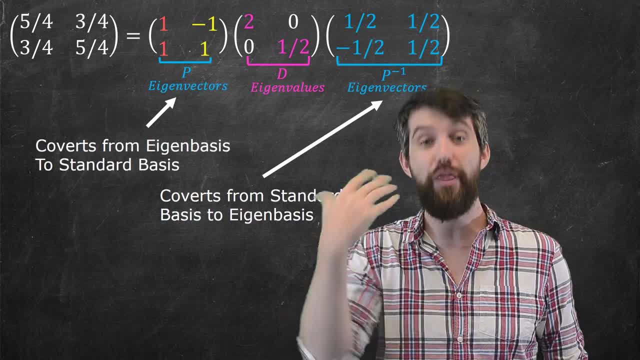 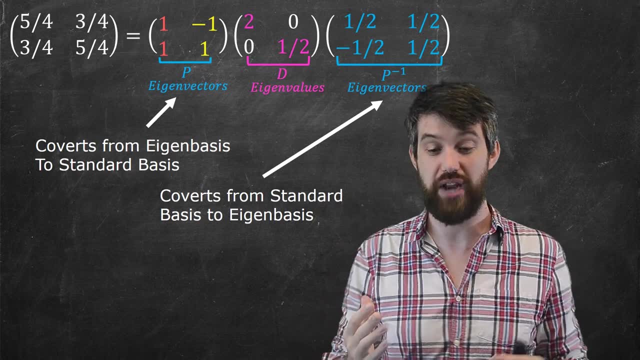 If that's what the p does, well, what about the p inverse? The p inverse goes the other way around. It takes vectors written in the standard basis and rewrites them in this eigen basis, The basis of eigenvectors that I've chosen in this particular order. Note, by the way, that there's several. 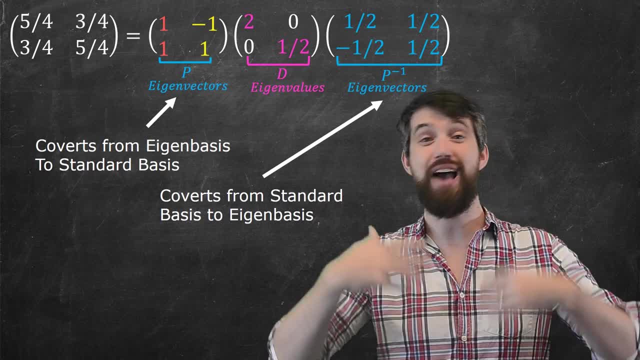 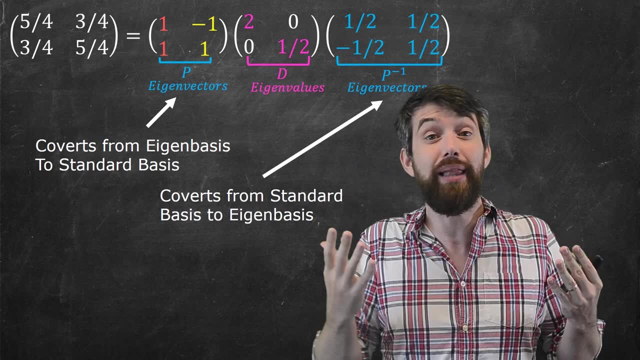 choices for diagonalization. I could take this 1- 1 and say have 2, 2 instead. That would be perfectly fine. I can permute the order of them, so the exact presentation of these is not unique, But nonetheless I have a basis of eigenvectors and I'm going to apply it in this. 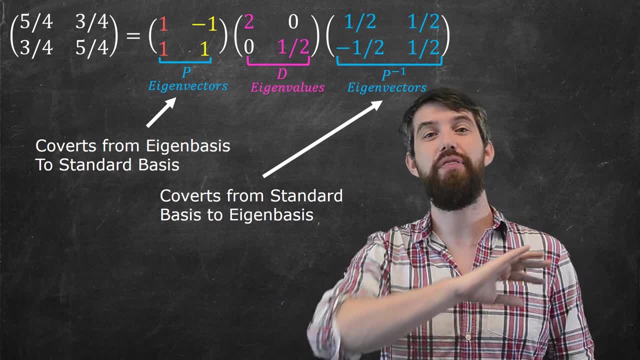 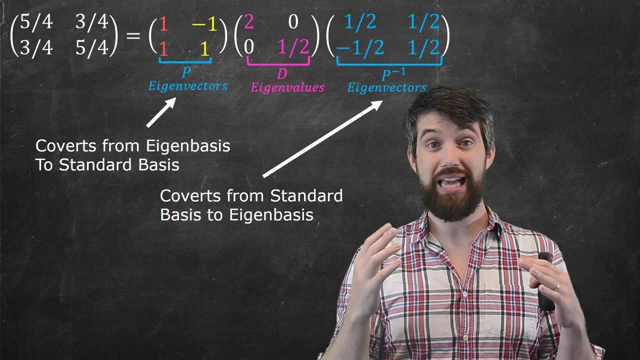 particular case. Also note: you can't always do this. It's not the case that you can always find a basis of eigenvectors. That's going to be a big topic for us moving forward. Alright, so now when I look at what's going on this, three different matrices multiplied are three different transformations. 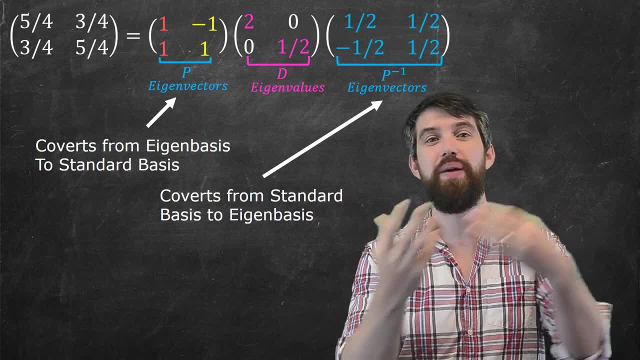 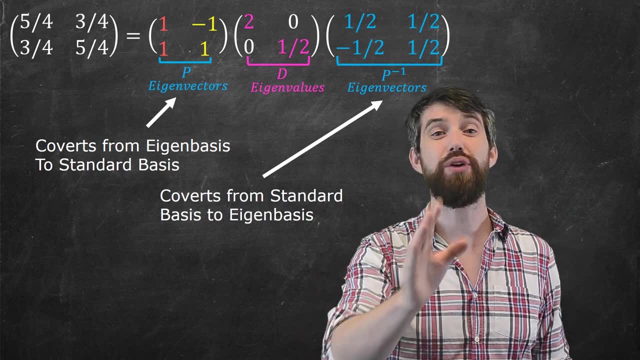 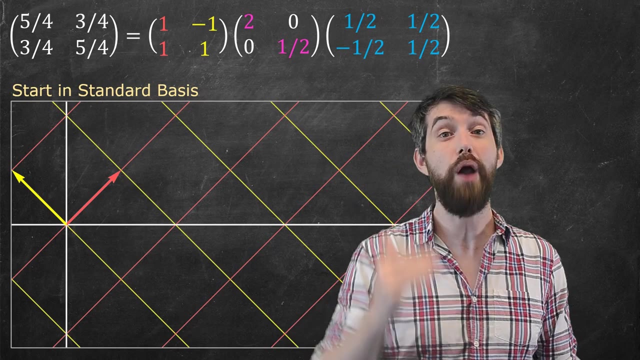 The p inverse is this one that's going to convert it from the standard basis to the eigen basis. Then I do something Diagonal and finally I convert back into the standard basis. So let's trace it geometrically Now. this is indeed the standard basis. For example, the one eigenvector is 1: 1 and it's sort of written. 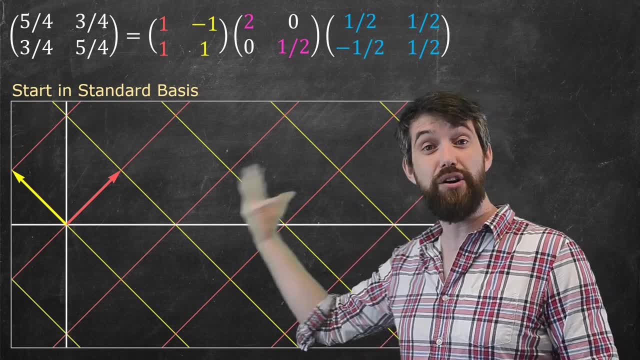 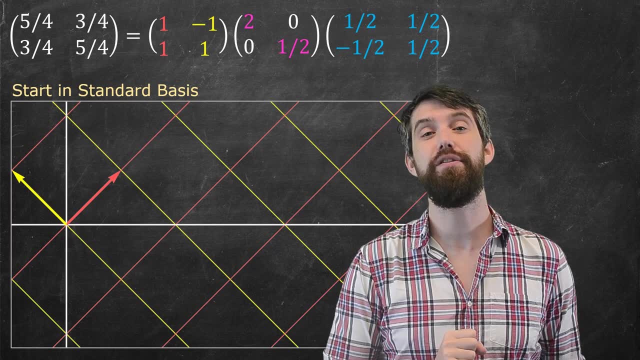 in the way you would write it in the standard basis, And I've given this entire grid system based on these two different vectors, But it's all written in the standard basis. Now I'm going to go and apply the p inverse matrix And what this does is it converts it to the eigen basis, The basis. 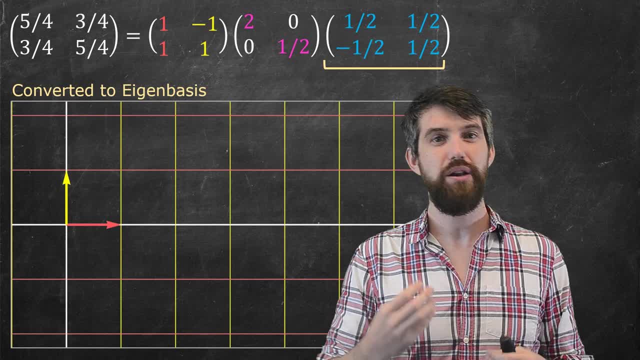 that is represented by the p inverse matrix. Now I'm going to go and apply the p inverse matrix And what this does is it converts it to the eigen basis, The basis that is represented by the different eigenvectors. Now notice from the perspective of someone living in the eigen basis. 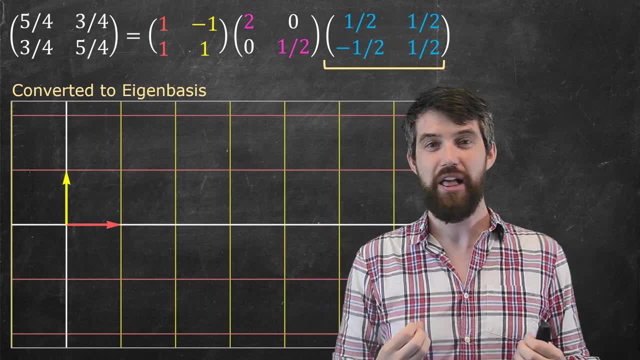 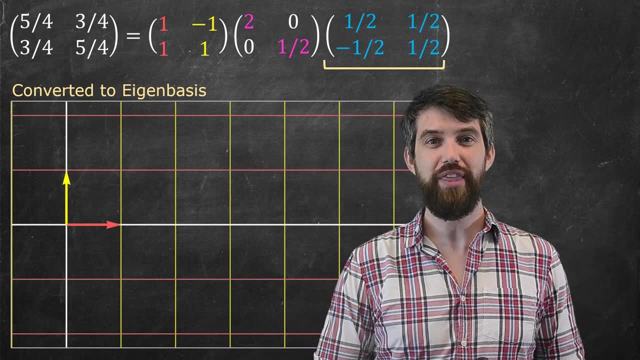 Somebody who spent their whole life hanging out in this particular basis. This is how they would draw it. It looks like the standard coordinate system, but it's not. It's how someone in the eigen basis would think about it. This one step to the right denotes go one along this particular eigenvector. 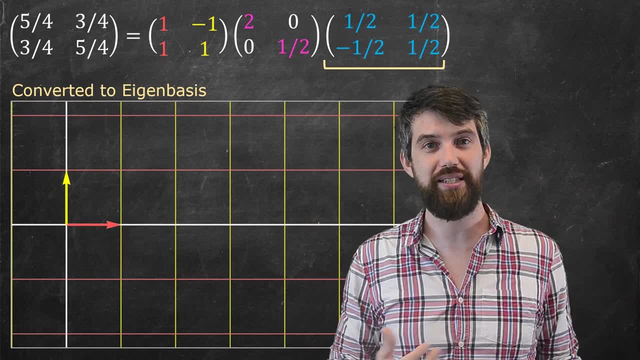 Alright. Well, now that I'm hanging out in the eigen basis, where everything looks really nice in the perspective of someone living in the eigen basis, I'm going to go and apply the p inverse matrix. Now, notice, from the perspective of someone living in the eigen basis, I'm going to apply my d matrix. 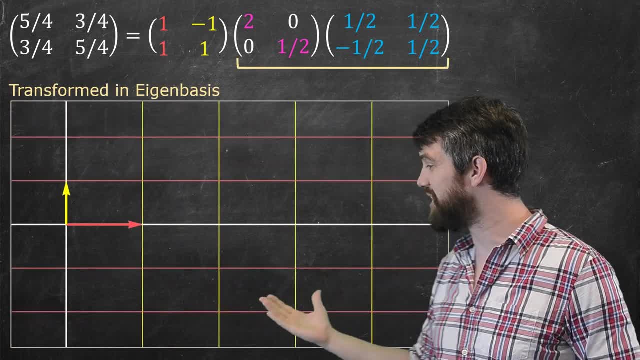 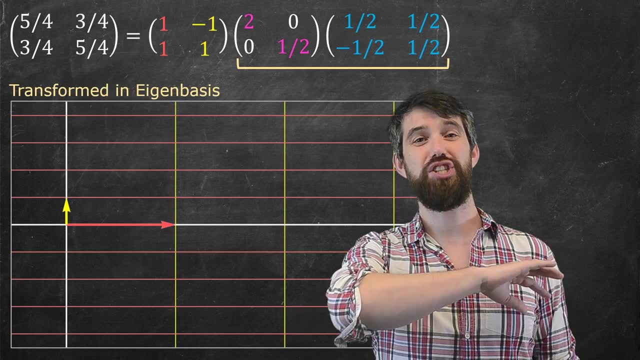 My d matrix is diagonal, so it's really easy to see what happens. It's just going to be this stretching factor by two horizontally, This compression factor by a half vertically, As in my transformation is just a diagonal one. when I'm in the eigen basis, I'm going to have to multiply. 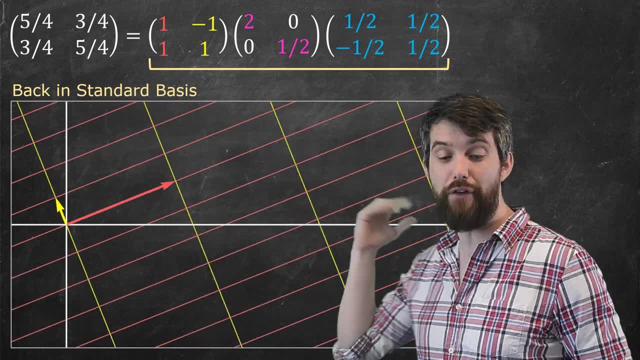 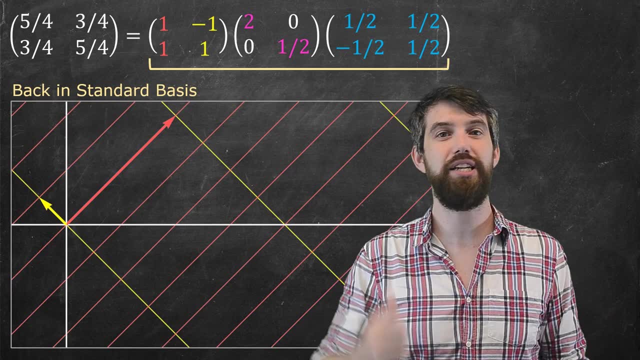 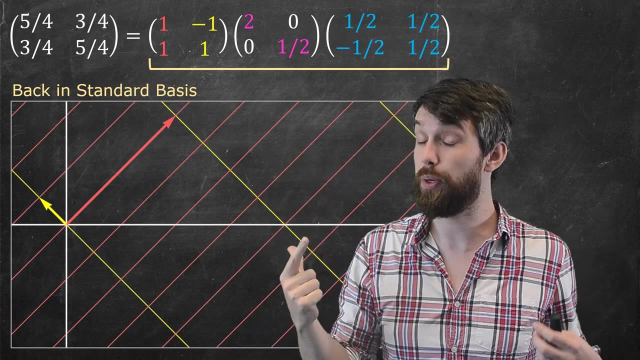 by my p, and so that's going to convert me back into the standard basis. Off I go and out. I get to this result that we've seen this output before. So what we have is these three stages: Number one: convert from the standard basis to the eigen basis. Number two: transform diagonally, which is